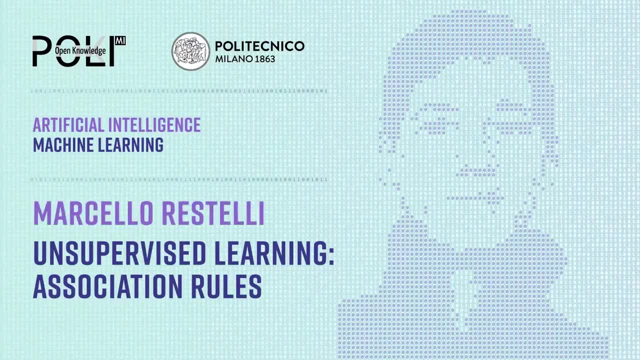 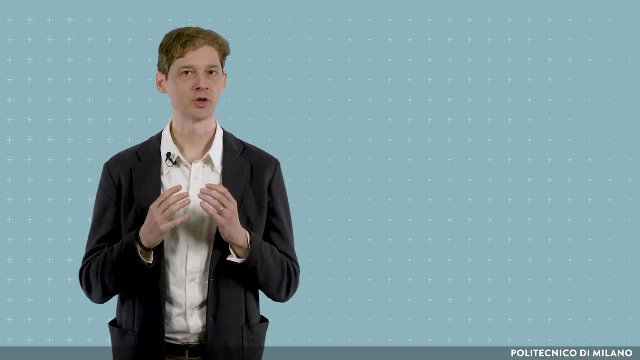 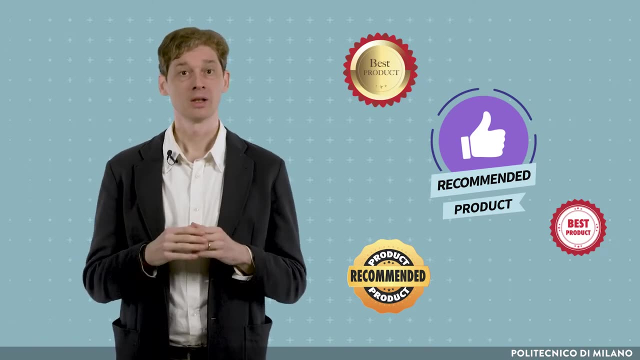 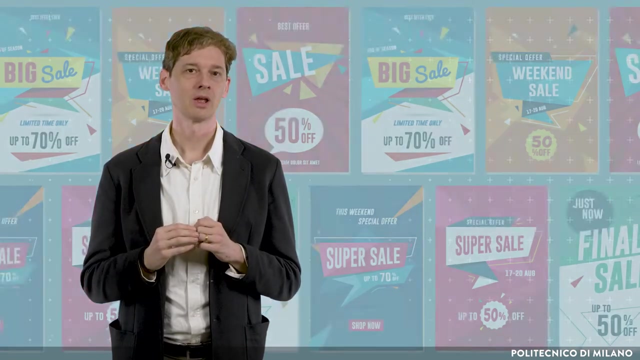 If you have done any online shopping, you have undoubtedly seen recommendations pop-up saying things like people who purchase this and that also purchase this, and that These suggestions are the result of a market basket analysis aiming at identifying frequent shopping habits. The goal is to increase sales by simplifying additional purchases for the customers. 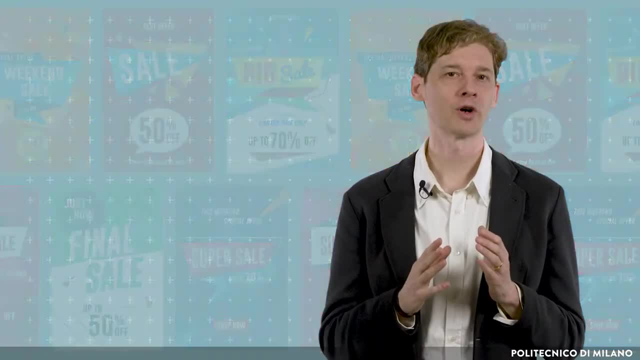 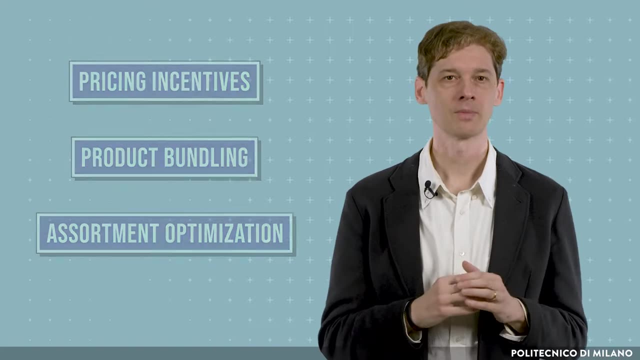 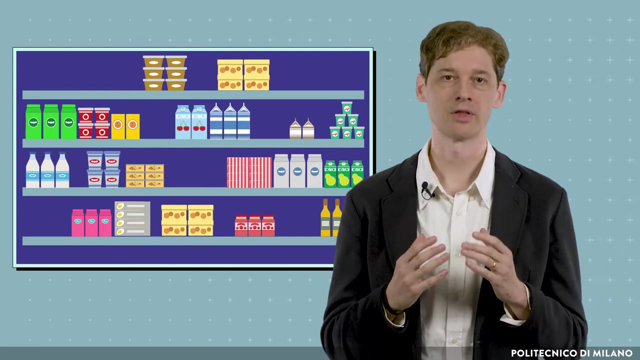 Besides cross-selling, these analyses can be exploited to offer pricing incentives on related products, to create product bundling and to make assortment optimization In physical store. such analyses provide suggestions on how to place products on the shelves to mutually promote their purchase. 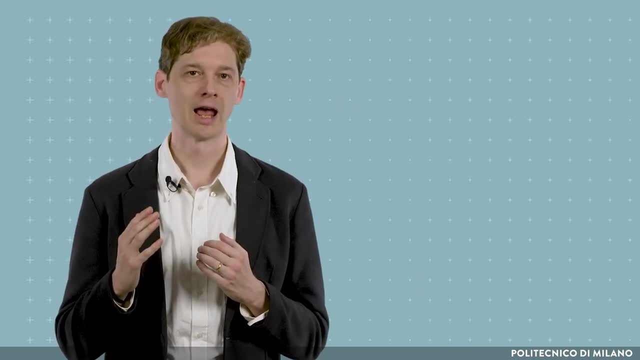 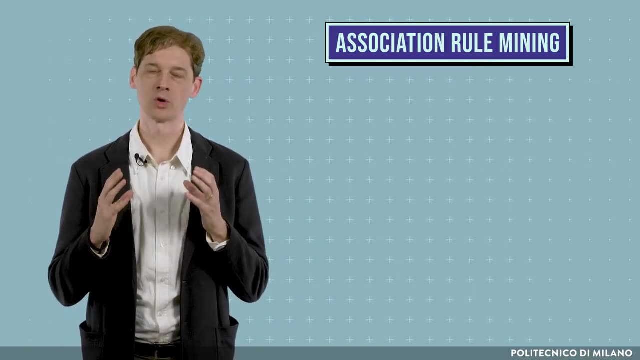 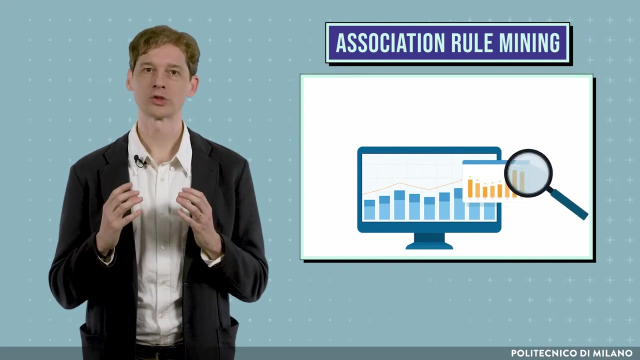 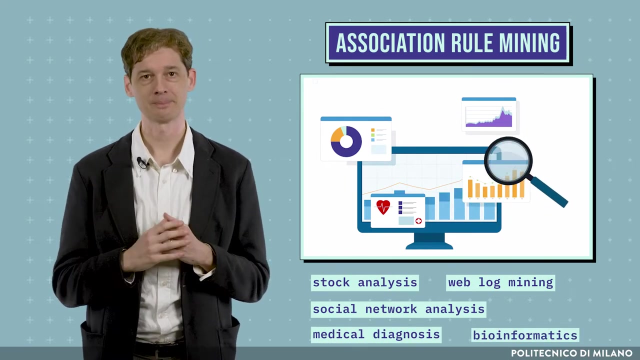 This kind of analysis is carried out using unsupervised learning algorithms called association rule mining. An association rule describes a relationship between variables or objects in a data set. In addition to market basket analysis, association rule mining can be used for stock analysis, web log mining, social network analysis, medical diagnosis, bioinformatics, etc. 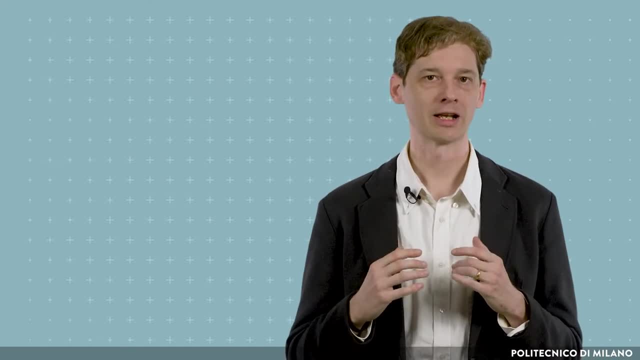 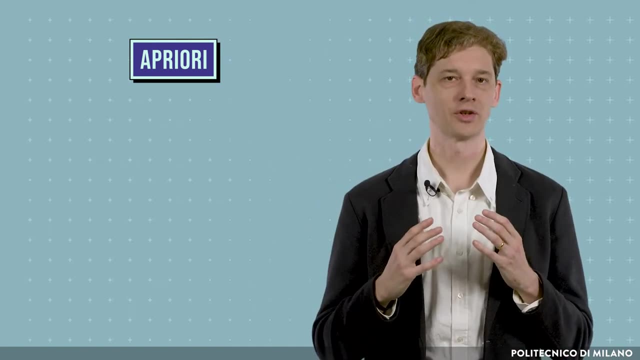 One of the oldest and most frequently used algorithms for discovering association rules is called Apriori, Apriori, Apriori, Apriori. Up to now, Apriori was designed to operate on data sets containing transactions such as point-of-sale transaction, which represents items bought together in a single basket by 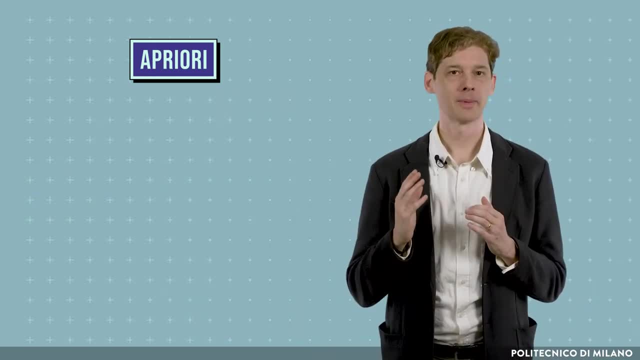 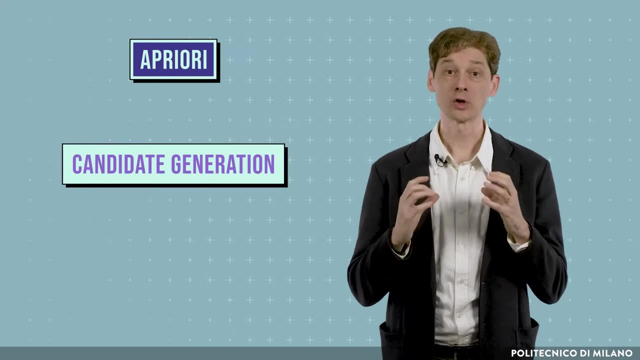 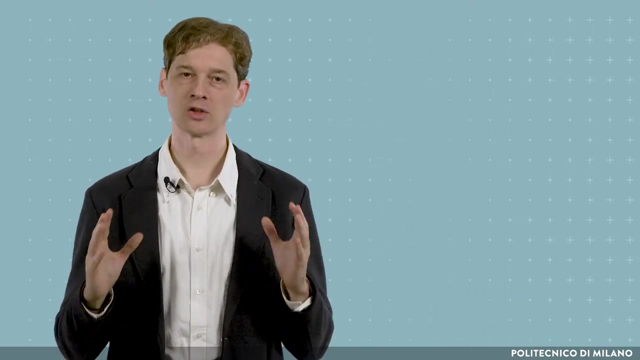 a customer. Apriori uses a bottom-up approach in which frequent subsets are extended one item at a time- a step known as candidate generation- and groups of candidates are tested against the data. The goal of this phase is to generate all subsets of items with a number of occurrences. 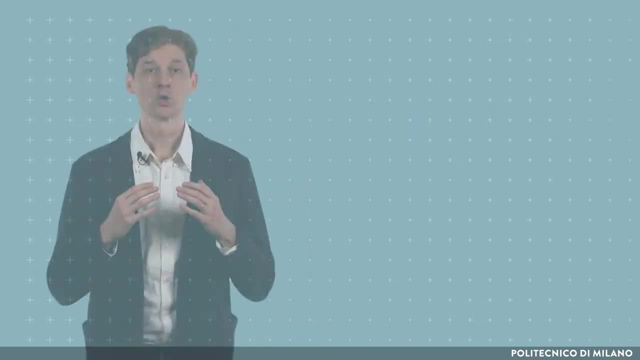 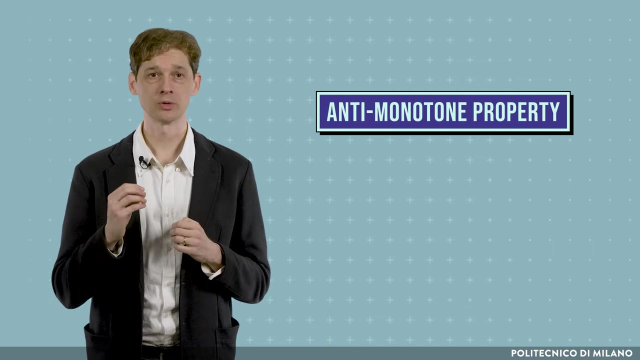 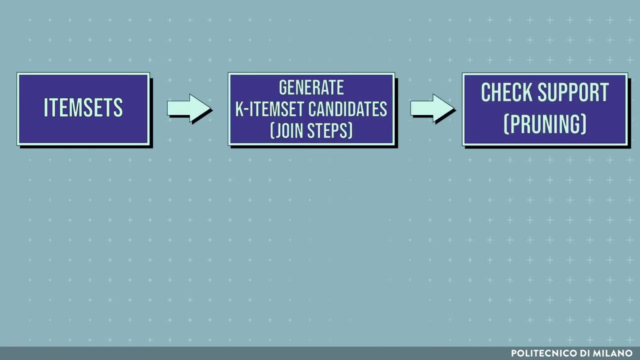 larger than the minimum support threshold. Using Apriori threshold To improve the efficiency of the generation of the frequent item sets. Apriori exploits the anti-monotone property, which helps to reduce the search space. According to the anti-monotone property, all subsets of a frequent item set must be frequent. 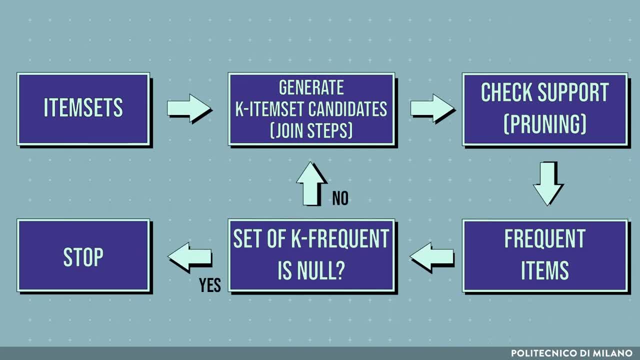 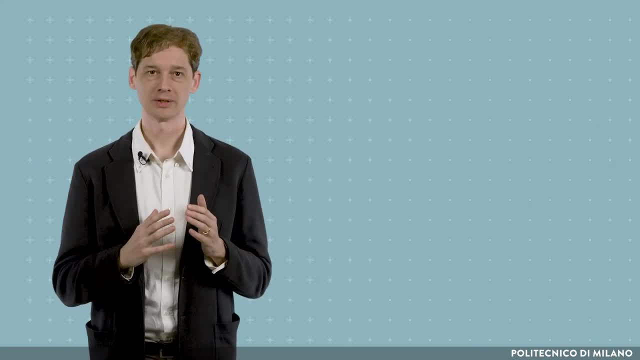 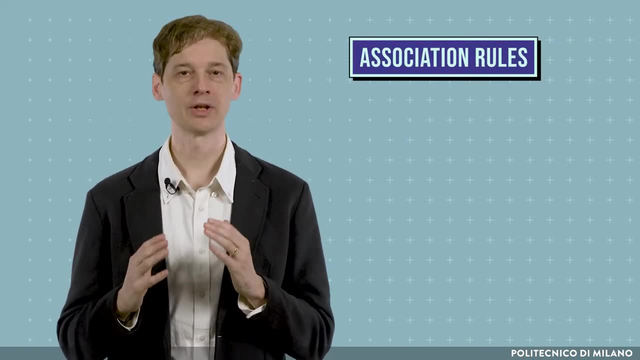 and if an item set is infrequent, all its supersets will be infrequent. Apriori terminates when no more candidate sets can be generated. Once the frequent item inserts are determined, the most prevailing association rules can be created and used to benefit the business. 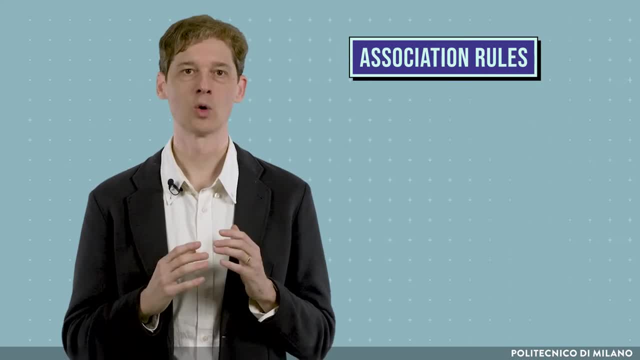 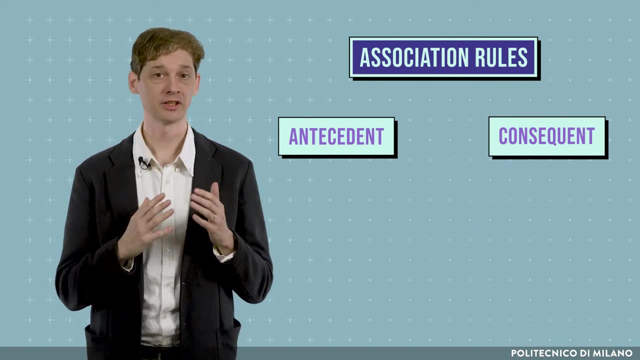 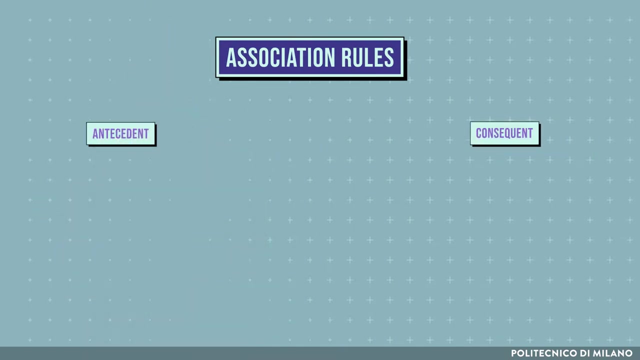 Each rule is composed of two different sets of items called the antecedent and the consequent. The meaning is that when the items in the antecedent are in a transaction, then we expect to find these items also in the consequent. 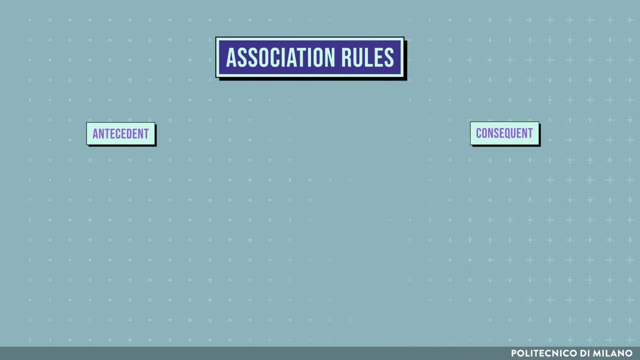 For instance, considering the supermarket domain, a rule could be: if butter and milk and bread are the antecedent and milk is the consequent, the rule means that in a basket containing butter and bread there is a high probability of finding milk too. 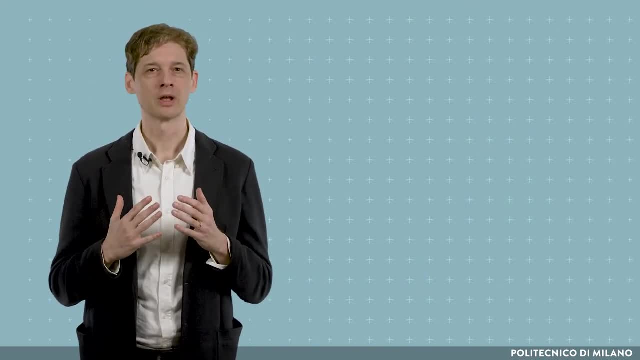 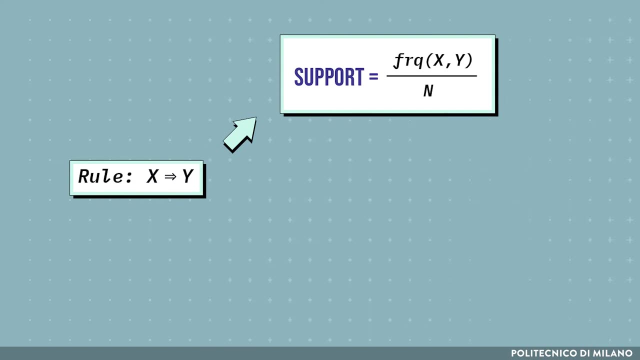 When assessing the power and usefulness of association rules, some key metrics are considered: Support: count: how often we can find items together in the same basket. Confidence: how often one or more items go into a basket when other items are already there. Lift: how more often two groups of items occur together than expected if they were independent. 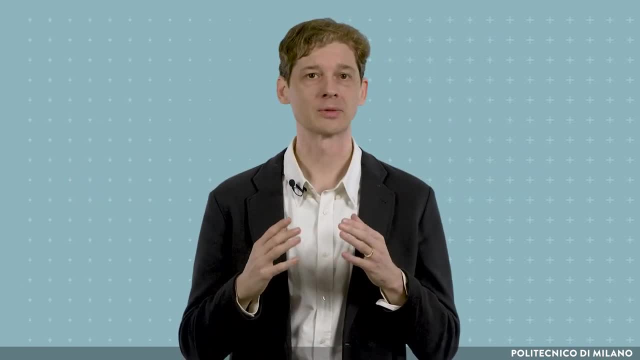 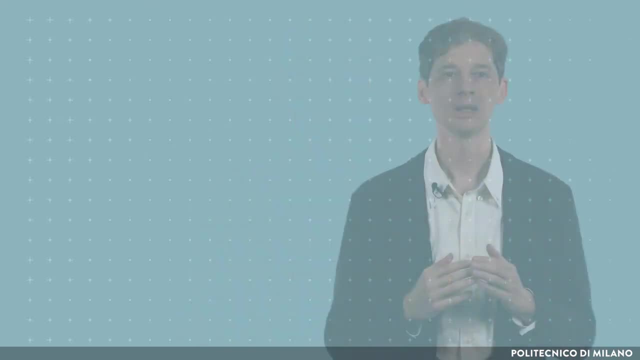 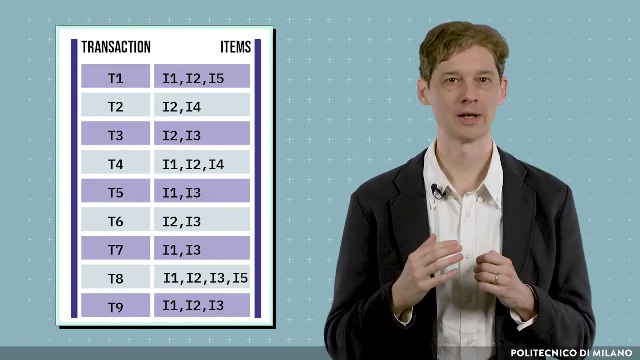 to each other. A powerful rule is expected to meet a minimum threshold of support and has high enough confidence or lift for practical purposes. Let's see now how it works with another example. In the table we see a set of nine transactions and for each one we have the items contained. 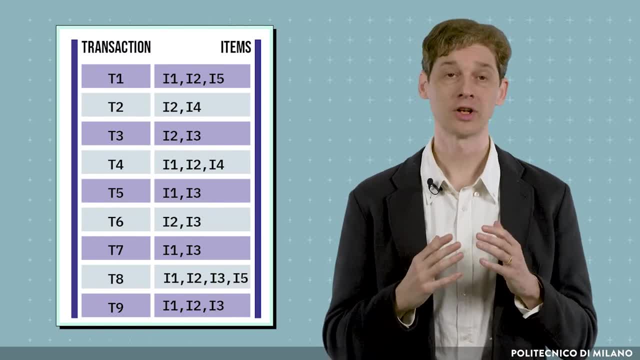 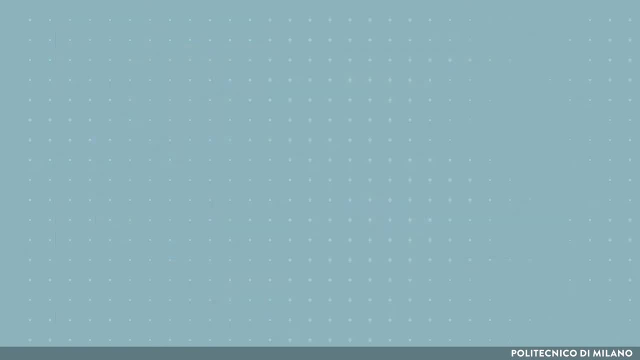 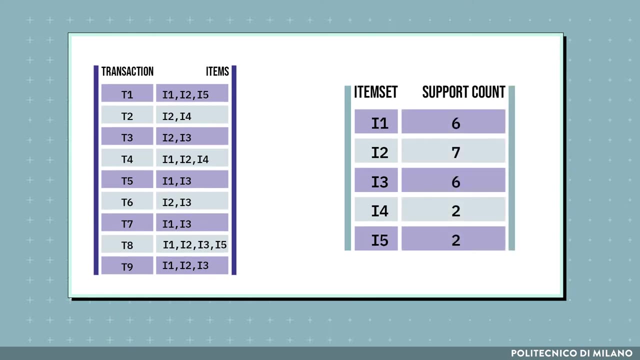 in each of them, We assume to be interesting rules, with a minimum support count equal to 2, and a minimum confidence of 60%. The first step is to consider each item present in the dataset candidate set and to compare its support count with the minimum support count threshold. 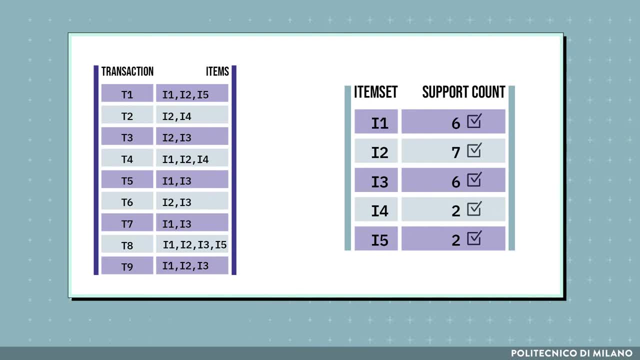 In this example we can see that all the items are frequent enough. In the second step, starting from the frequent items that are identified during the previous step, we consider all the items set with two items and again we test if they are frequent enough. 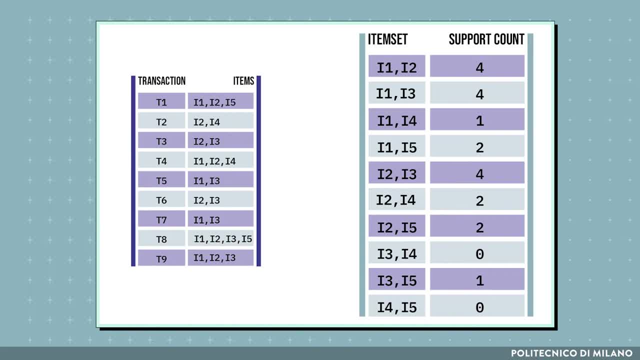 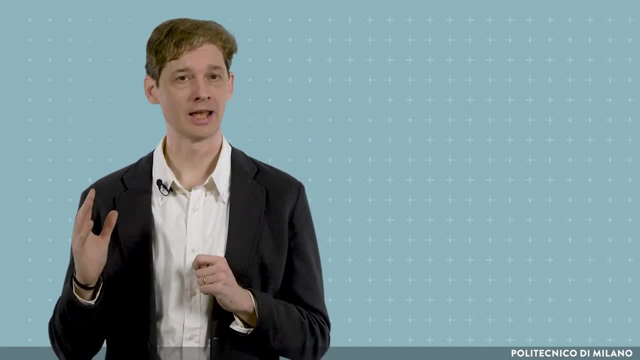 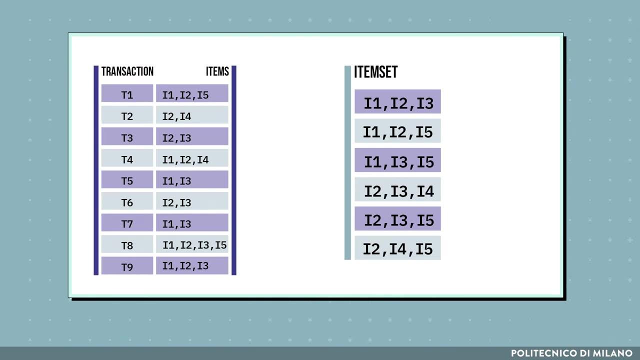 In this case only six of the original ten item sets are frequent. Starting from these item sets, we generate the candidate sets with three items. These new candidate sets are frequent only if all the subsets of them are frequent. So for instance, the item set I1, I2, I3 may be frequent as the item sets I1, I2, I1,.